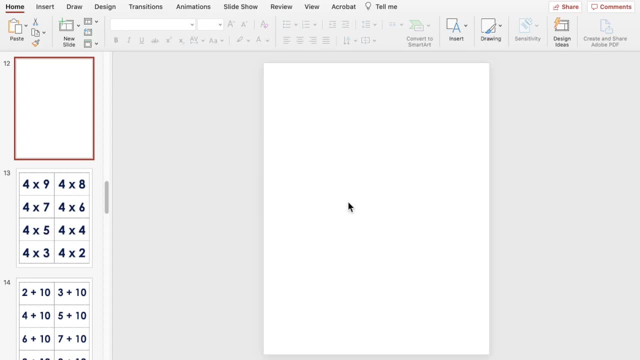 to know how to set up your pages on PowerPoint. check out any of my videos- numbers 1 through 15- in my 30-day back-to-school math resource challenge, and I break down how to set up your page, as well as, when you're finished creating your printable, how to save it and export it as. 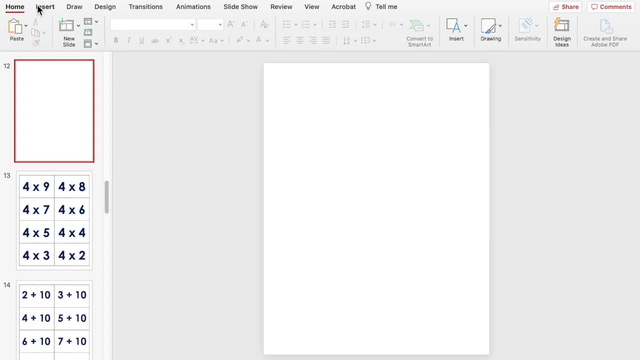 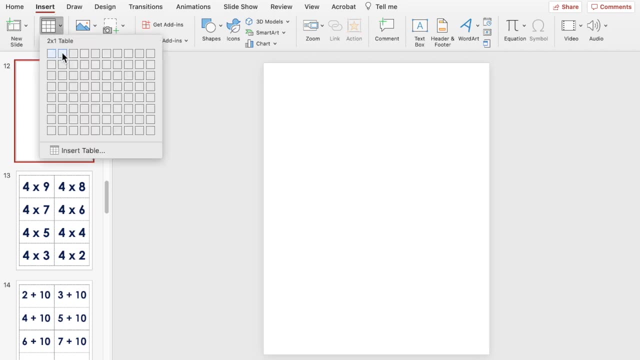 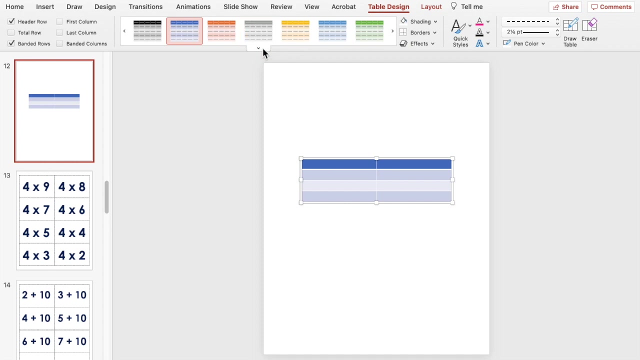 a PDF. So, to create this first page, you're going to start with a simple table. so I'm going to go to insert table and then I'm going to have two columns and then four rows of those columns. so this is the table that pops up. so I'm going to go to table design. 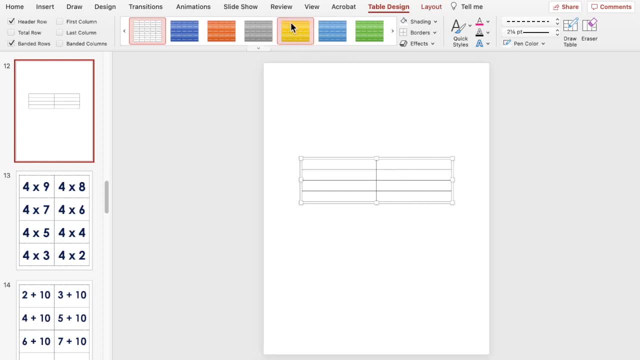 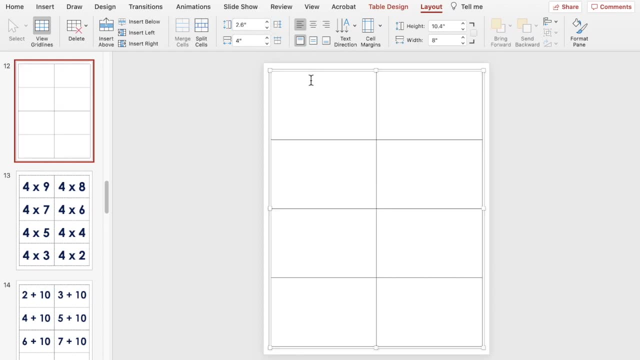 and then go to the blank, no style table and then switch my tab to the layout tab and increase the size of the cells. all right, so there is the base of our flashcards, and then we're going to insert a text box to add in whatever content that you want your students to work on. you're going to 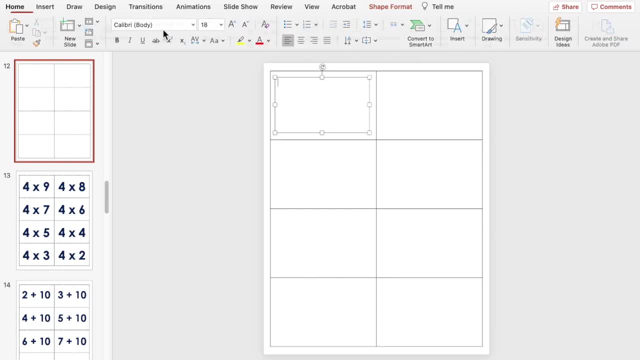 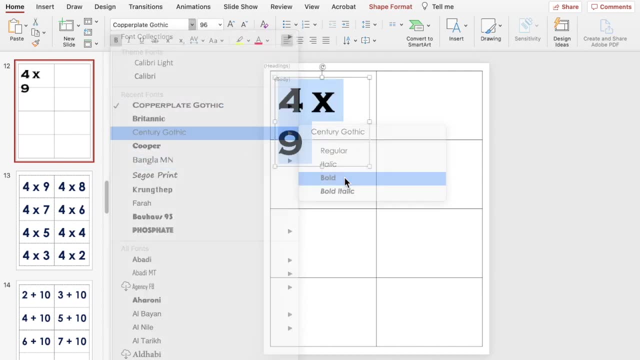 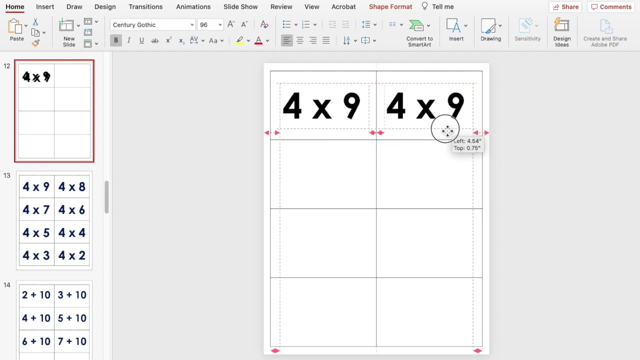 create that text box and we're going to go to home to look at the font- let's go with my favorite century gothic fold- and then we're going to center it and there is your flashcard. so I'm going to duplicate that and move this over and make. 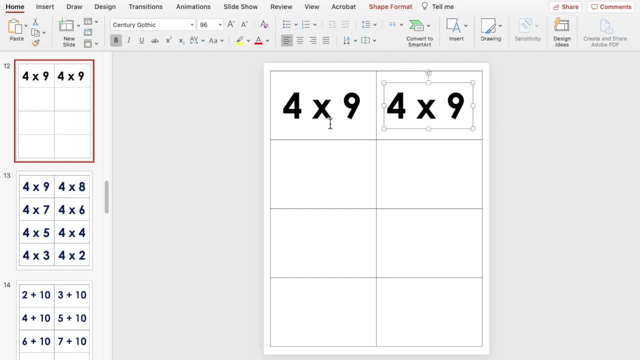 sure it's aligned. and then I'm going to select the one I just did and the first one, and I'm going to hit command D on my keyboard or hit control D if you have a PC- I have a Mac- and bring that down and make sure it's aligned and then hit command D again and 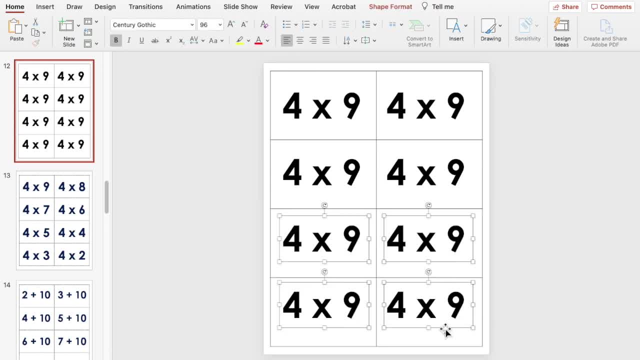 then once more- and I want to move these down slightly- so I selected all of them so I can bring them down. now I'm going to go in and change the numbers, so I did this before- let's do sixes- and I didn't realize I wanted to switch to six. so I definitely would recommend doing the first one as. 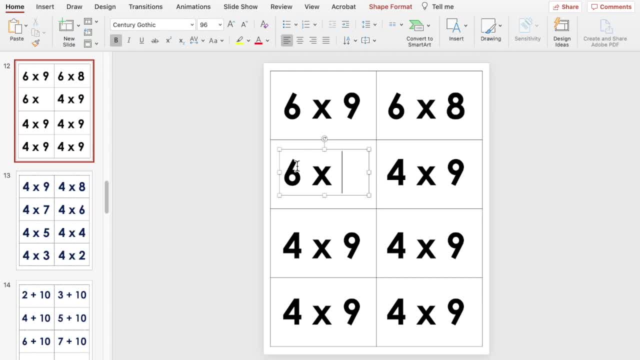 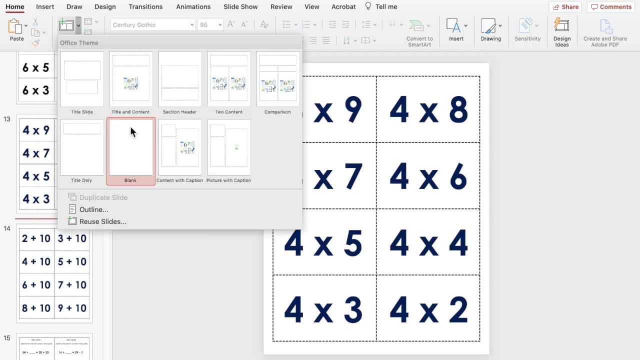 the six and then duplicating it, so you don't have to change both numbers for each card. and there you have your simple flashcards to practice multiplication. you can do the same thing with addition. so I'm going to insert a new slide here, the blank slide. you can do any of the operations you can do. shapes you can do. 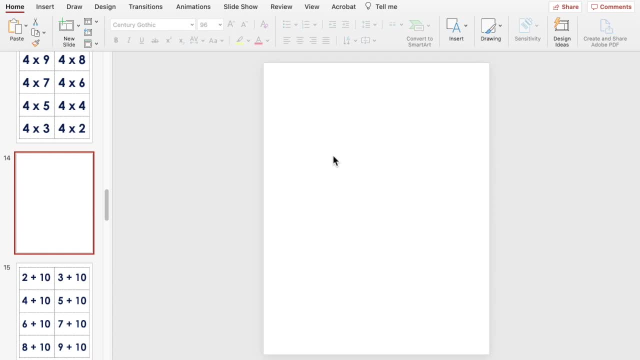 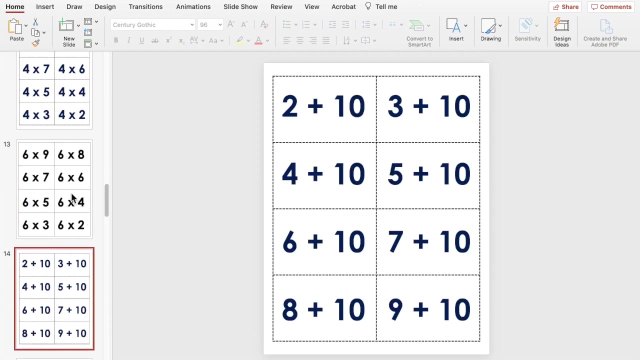 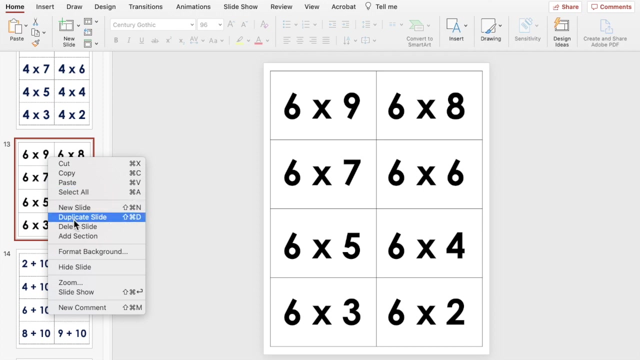 vocabulary words. it's not contained to math. you can do any subject- vocabulary and science. so actually I'm going to take the ones that we just created and, instead of creating a new slide, I'm going to duplicate the slide that we have. so I'm going to select that slide and then click right, click it and go down to duplicate slide and we're just 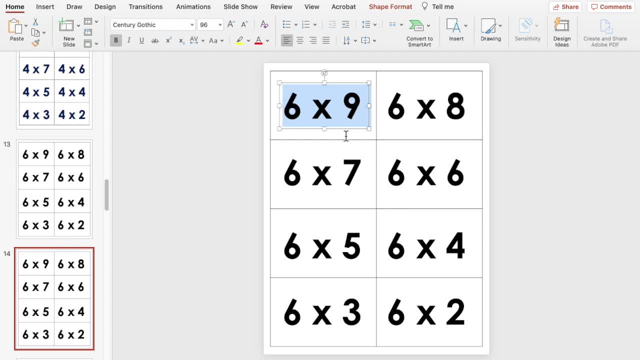 going to change these out to addition or we can do subtraction. so if I wanted to do 10 minus a number, decrease the font size so that they fit. I'm going to get rid of these down here instead of changing them individually and duplicate same thing that I did before. command E on my keyboard. 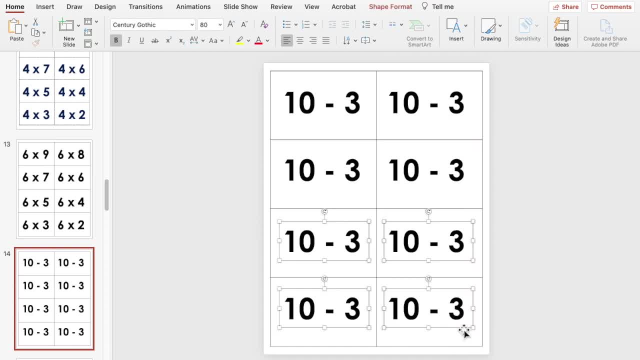 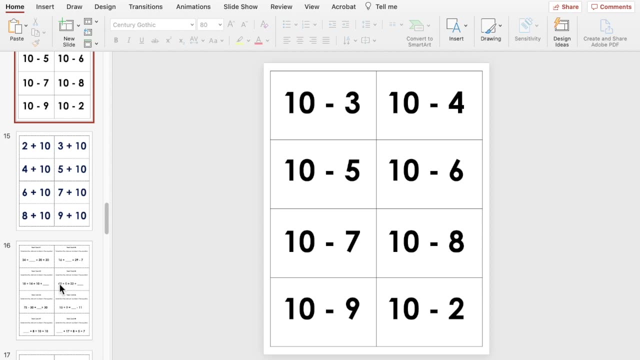 make sure they're more in the center and then go in and change my notes to numbers. so easily we switched it from multiplication to subtraction again. you can use flashcards for a variety of things. now I want to do. I want to turn my flashcards into task. 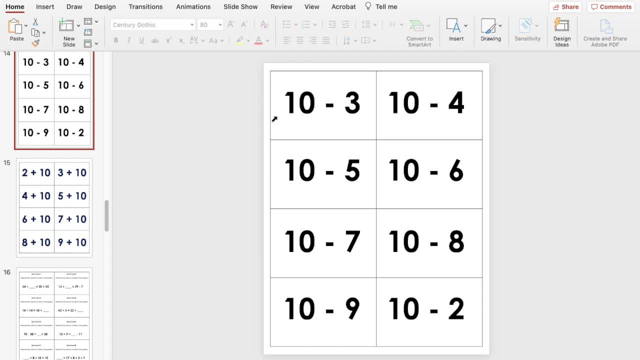 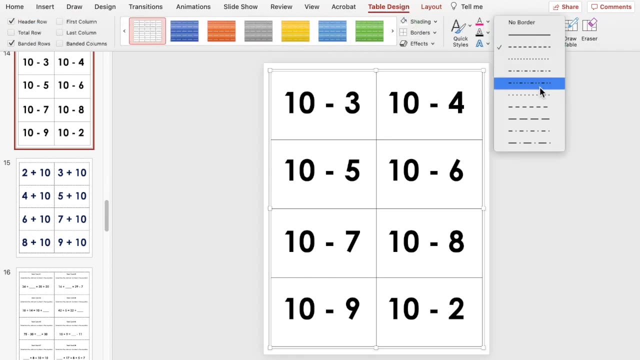 cards. oh, and let me show you how to change your lines to those perforated lines. so if I select the table and I go to table design and we click on lines, we can select whatever dotted perforated lines that you want and then click border and click all border. oh, let's bring that back. 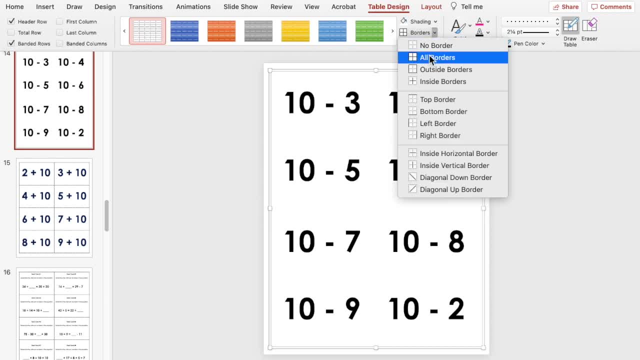 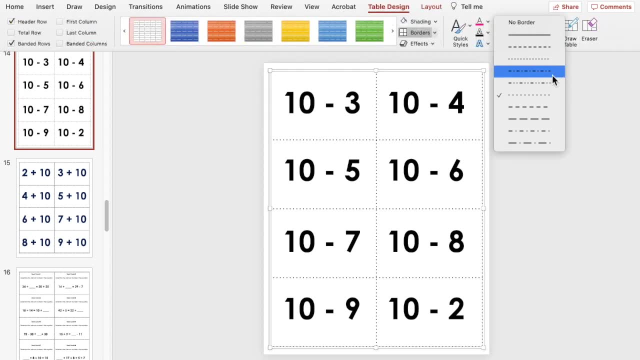 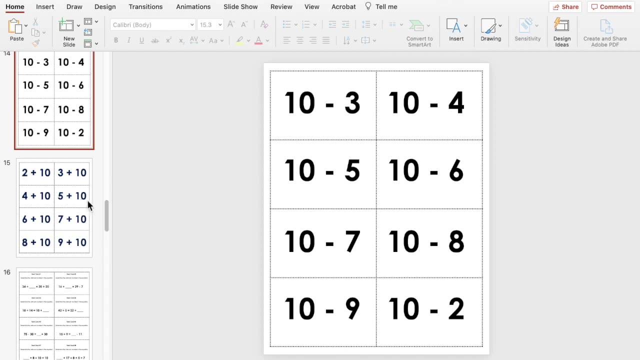 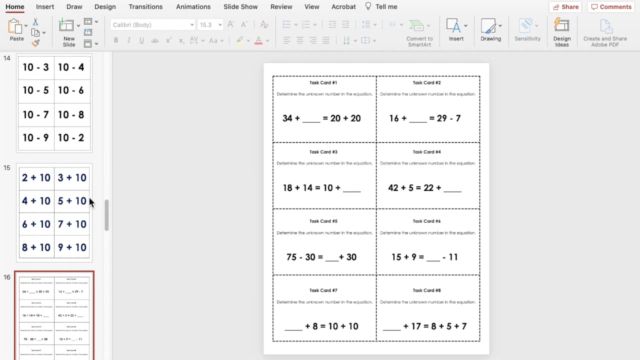 make sure your pen color is black and then go to all border and there are your dotted lines. if you didn't like those, choose the ones that you like. let's choose that one and then click all borders again. there we have our flashcards. now we're going to create task cards. same setup. 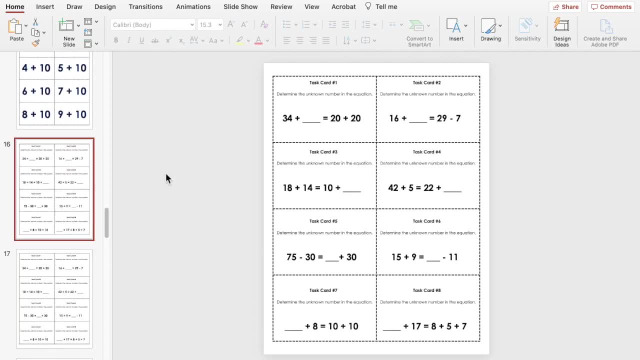 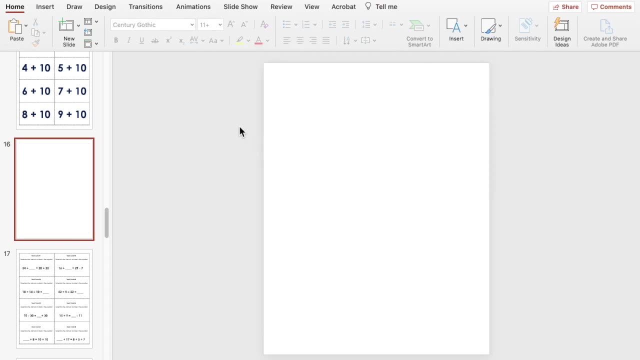 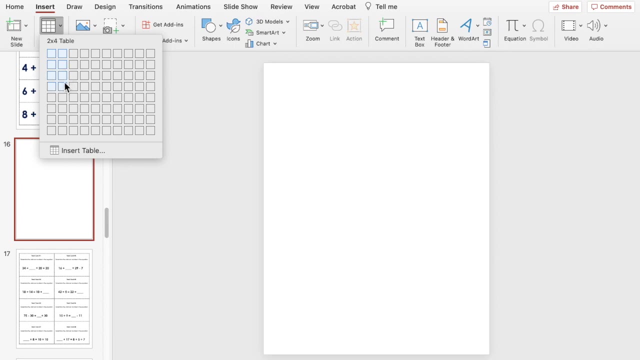 so I'm going to duplicate this page and delete. I guess I didn't need to duplicate it. I can create it. I could have created a new page but insert. we're going to go to insert and table and we're going to do two columns of four again and then we're- let's go ahead and change our lines here. 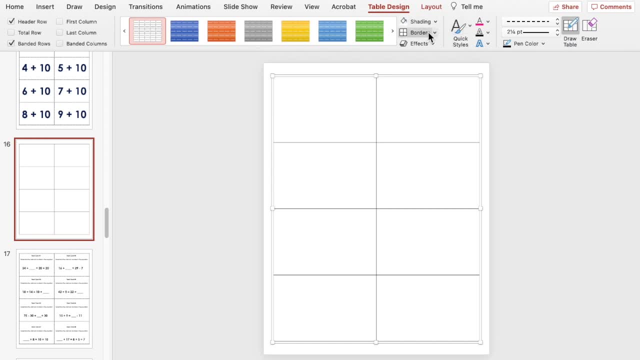 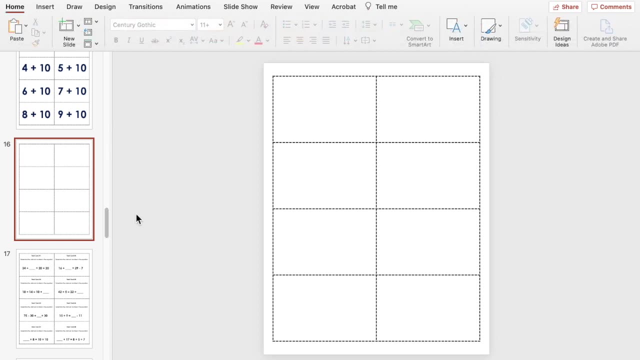 click our let's do these lines this time, these dashes, and then again click all borders. so now for what's inside. I want to. I'm gonna add in little text boxes for each part of the task card. so I want a title, one for my instructions and then one for the. 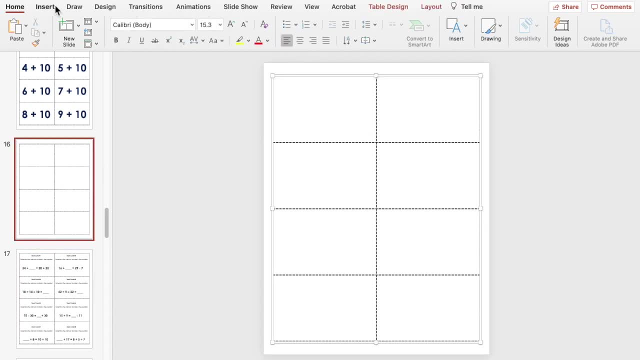 actual question. so we're going to go to insert, go to text box and we're going to type in what we want to call it so we can just say task card number one. if you're doing these for groups, you can separate it by color, like blue group task cards or group number one task cards. so I'm going to go to home. 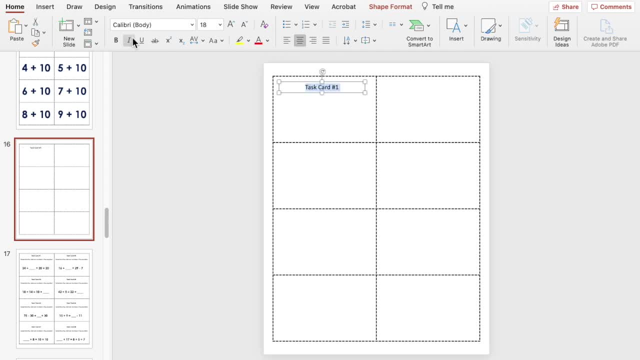 and center that and make it bold and then switch the font and you can add color here if you want. so task card number one. I'm going to duplicate that to write the instructions so that the task cards I'm creating are a, determine, the unknown number in the equation, and then I'm going to take the task card one again to duplicate control d or.